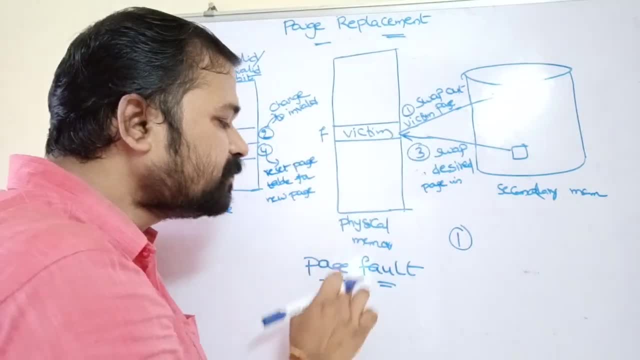 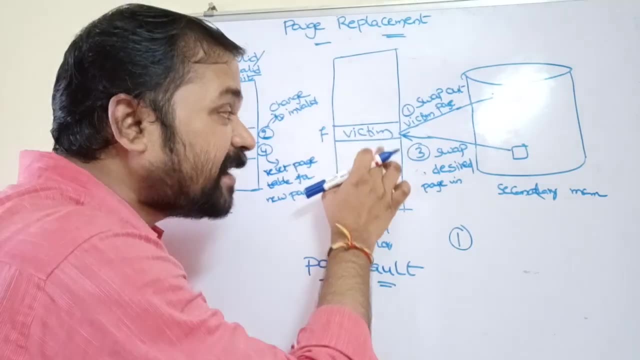 Swap out a victim page from main memory to the secondary memory and then now the main memory does not select a page from secondary memory, and after that we have Gl Tucker here and I make a fine connection between the main memory and the secondary memory. Next interface I will give: 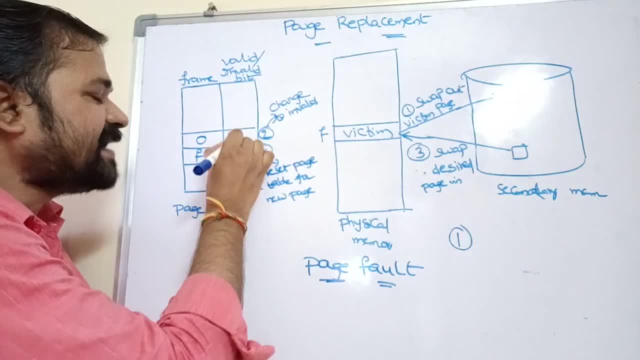 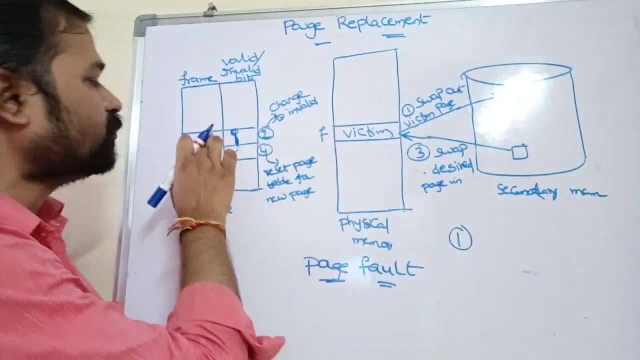 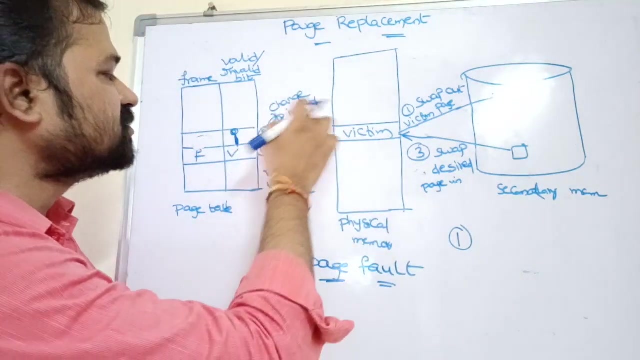 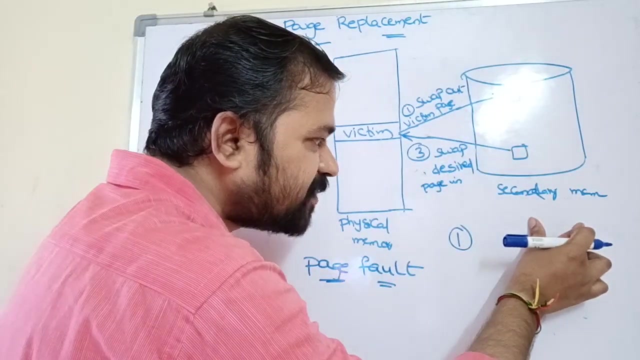 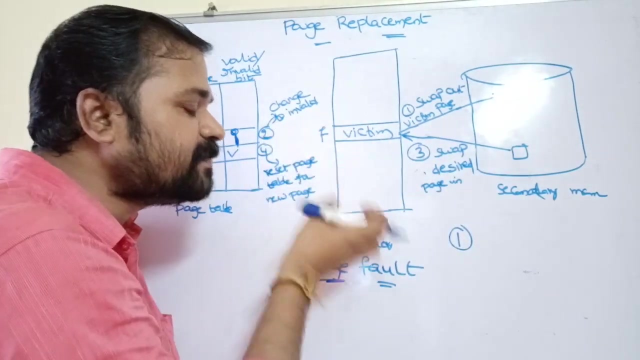 you is called NVU TikTok. We will have that estruct Here. you know we have this Его the required page from secondary memory to the primary memory. so swap desired page in. so now our main memory contains the corresponding page. and the last step is now the main memory contains the. 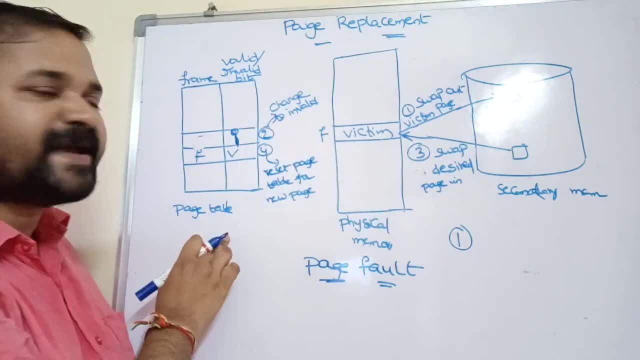 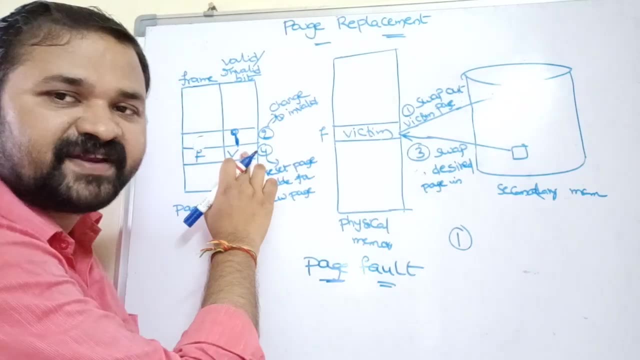 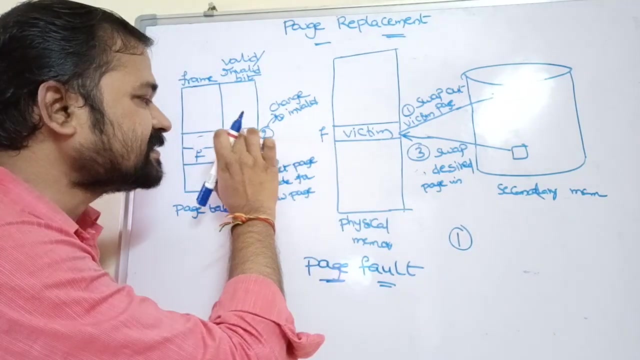 corresponding page so that information needs to be updated in the page table. so here we specifies that the corresponding page is available in the main memory. b stands for valid bit, i stands for invalid bit. so we specifies that the page is present in the main memory, whereas this i specifies. 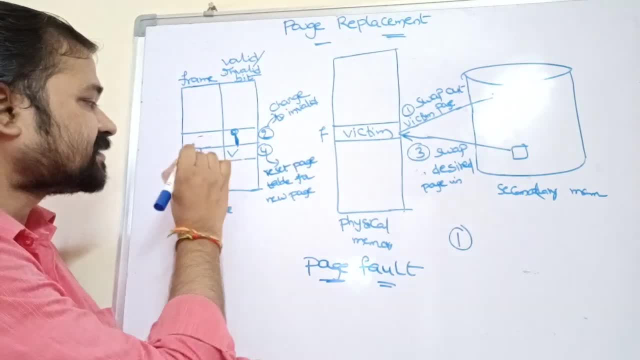 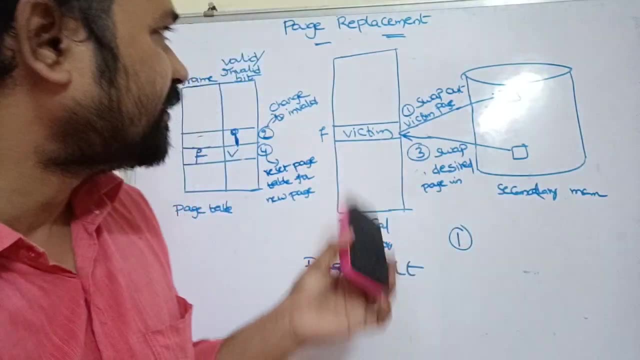 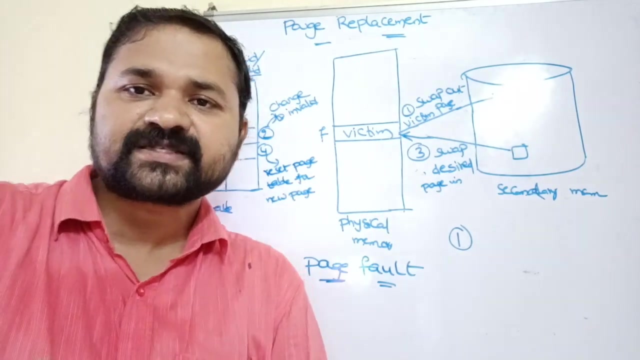 that the page is not present in the main memory as well, as we have to provide that frame number information also. that is nothing but f. okay, so this is about the page replacement. so totally, we have four steps so before. so whenever a page fault occurs, their operating system loads a page. 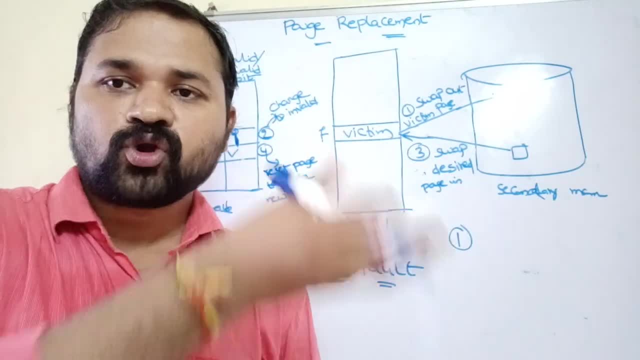 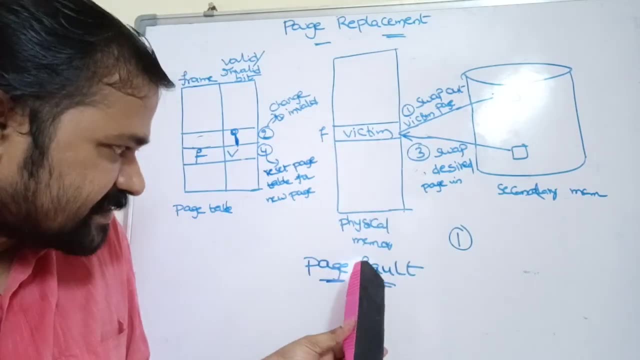 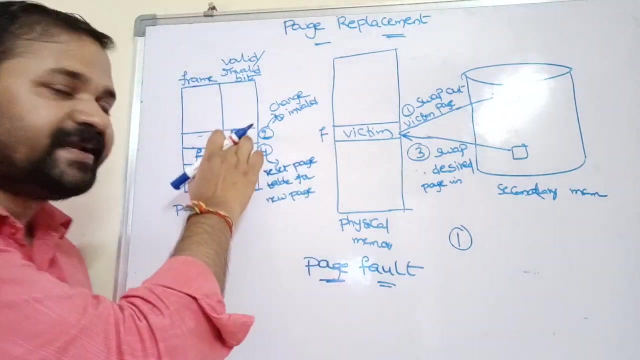 from secondary memory to the main memory. so, before loading into the main memory, what we have to do? we have to swap the selected page from secondary memory, from main memory, to the secondary memory. now, main memory doesn't contains that page, so that information needs to be updated here, as i, so i specifies that this page number, let us assume, 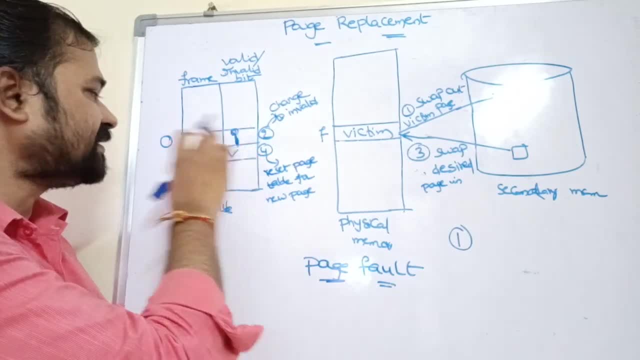 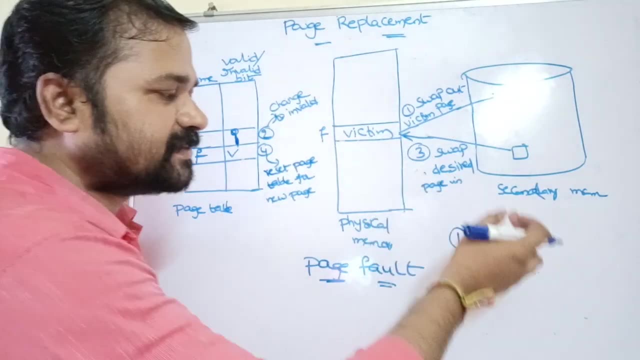 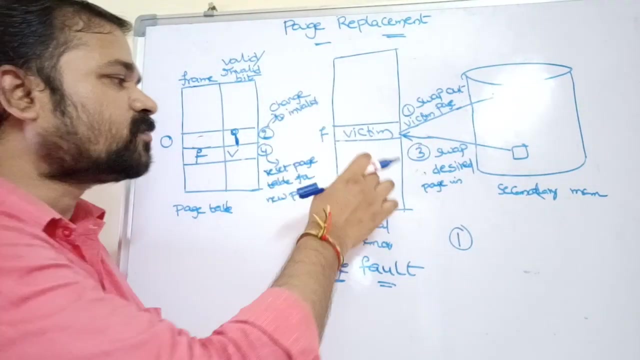 that here this page number is some zero. so this i specifies that page number zero no longer belongs to the corresponding main memory. okay, and after that the task here is move the load, the corresponding page from secondary memory to the main memory. now our main memory contains the corresponding place, so that information should be updated here by specifying. 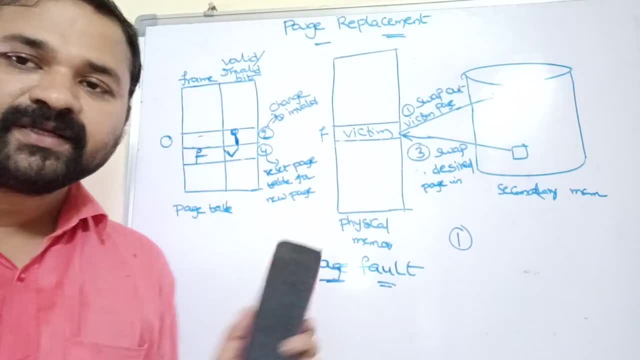 the frame number and value bit. so this is about what is the need of case replacement. now let's see about various space replacement algorithms.